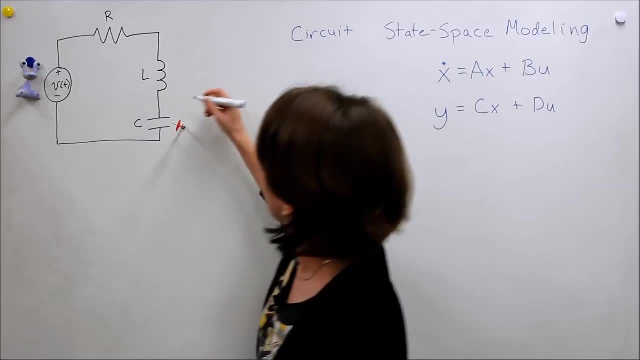 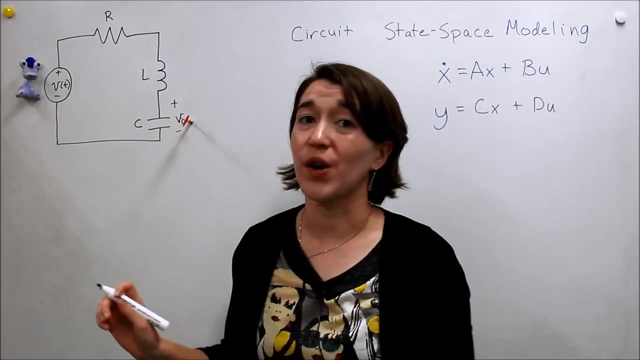 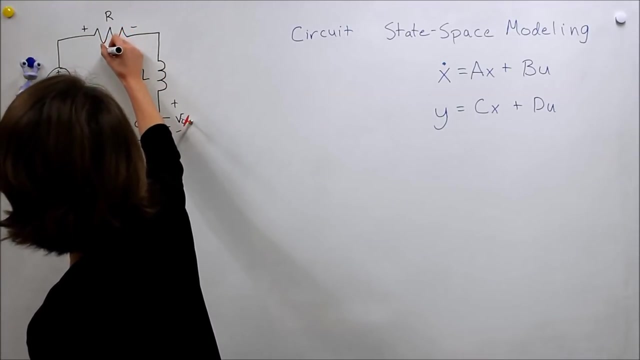 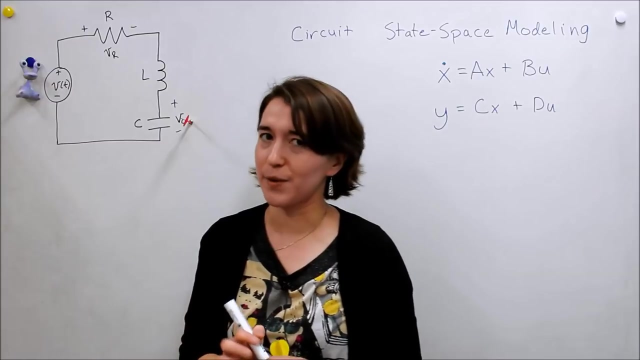 of our output. our target will be this voltage, so it'll be the capacitor voltage, Oops, VEC. And the other one will be the voltage over this resistor, So we'll call that well VR. And our input is Valerie. She's controlling our voltage here on the input, So let's model. 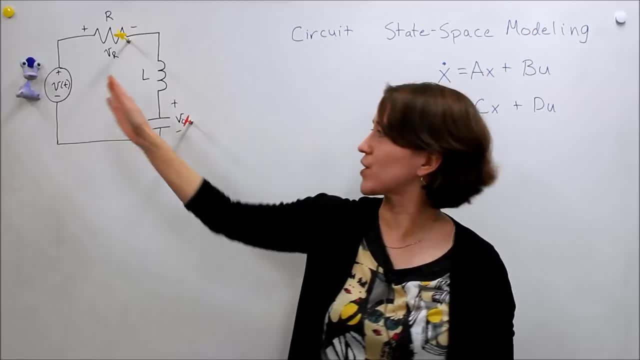 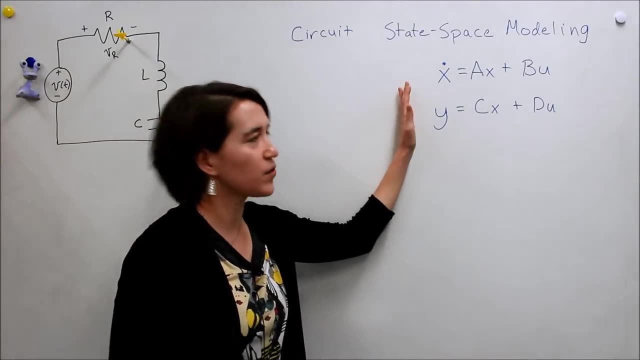 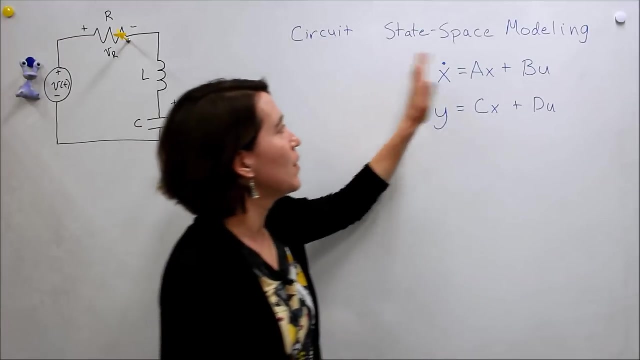 this system. Oops, sorry, This is our second output, so our output one and two. So let's model that, All right? And just to remind you, this is our standard form for state-space space modeling. If I say put it into state-space form, it means you need to find A, B, C, D and write. 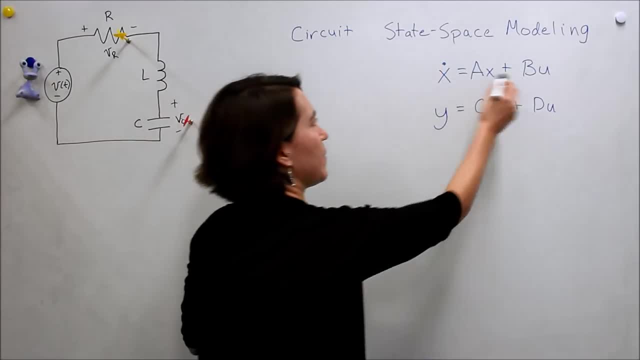 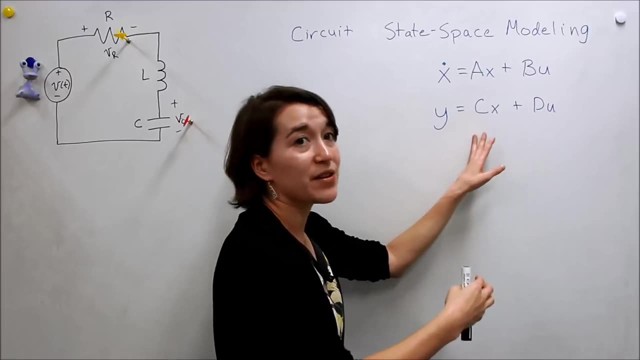 it in this form And as a reminder: A, B, C, D are all matrices. They might be one-dimensional or 1,, 1,, 2,, 2, but they are matrices. And then X and Y are and U are vectors, So where? 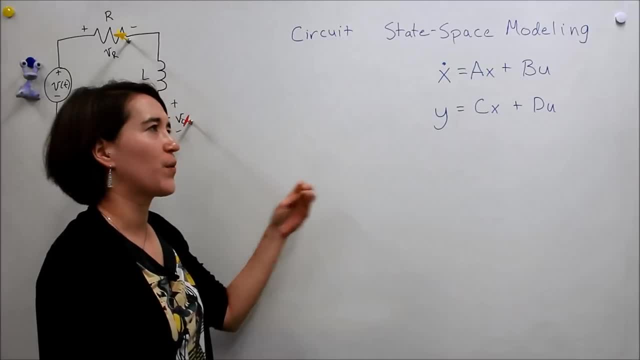 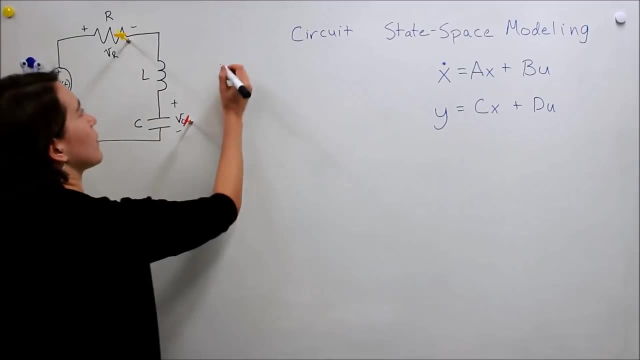 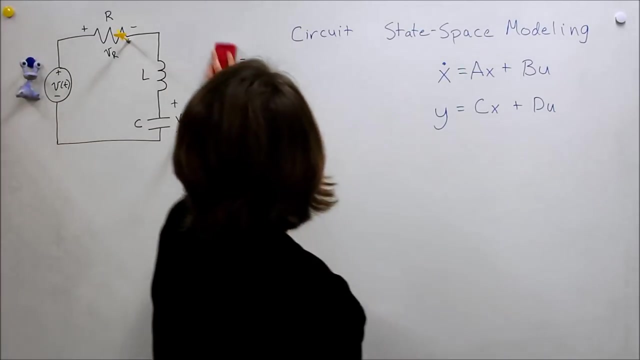 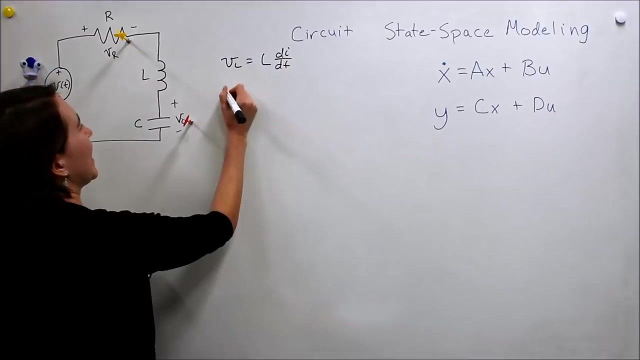 do we start on this? I'll give you my approach for working with circuits. If we remember the equation: for an inductor, we have V. sorry for a capacitor, Oh gosh, I always fail. this one I equals, oh no, it's V- equals L D I T. It goes: L D I D T. 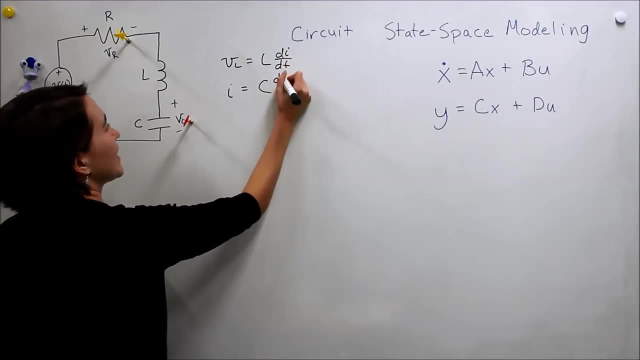 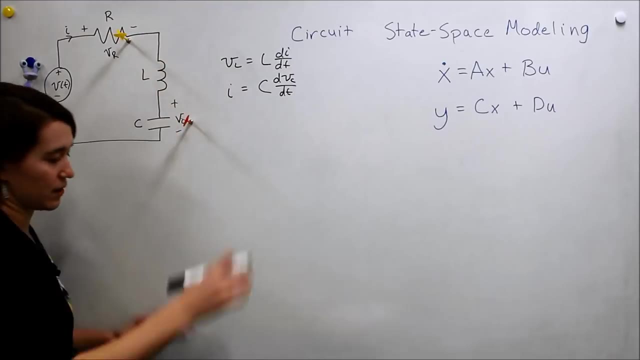 And I is equal to C, D, V, D, T. Okay, and here we're defining the current: the same through all of them and then each of these voltages. So these are our equations and we have this derivative. here We want to find a derivative. 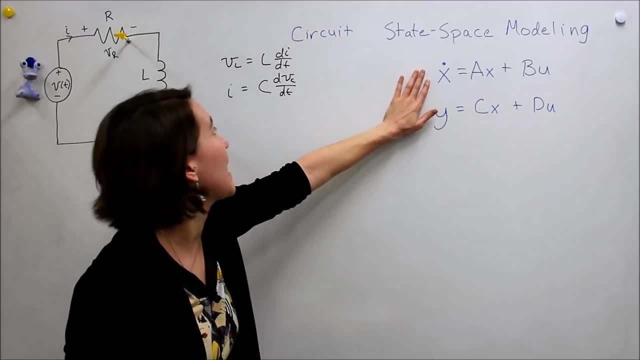 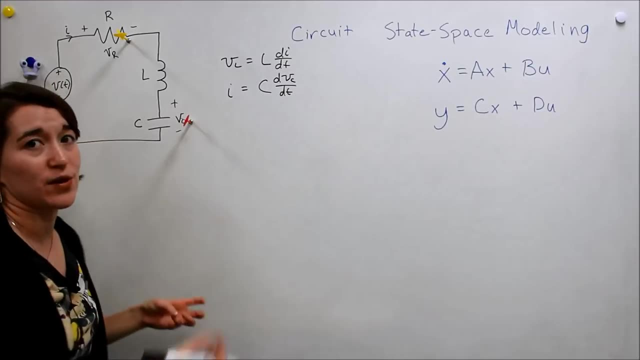 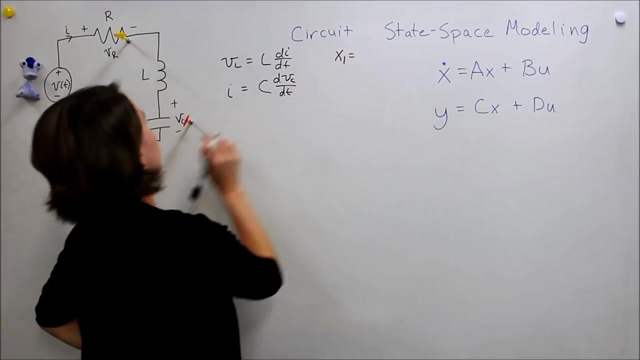 equation for each of these. so it makes sense that we name our states to be V, C here and I. So you get to choose which states, but you have to make sure you're capturing all the dynamics in the system. So in this case we're going to define. we'll say X1 is equal to this capacitor voltage. 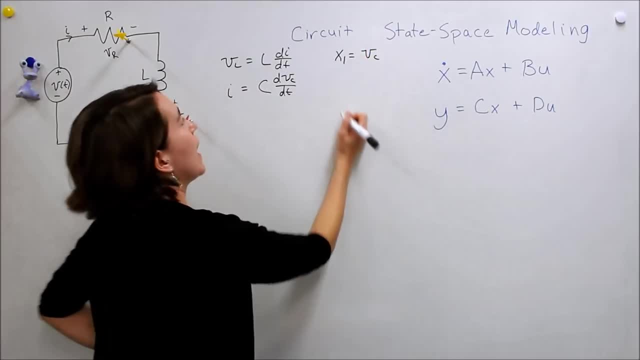 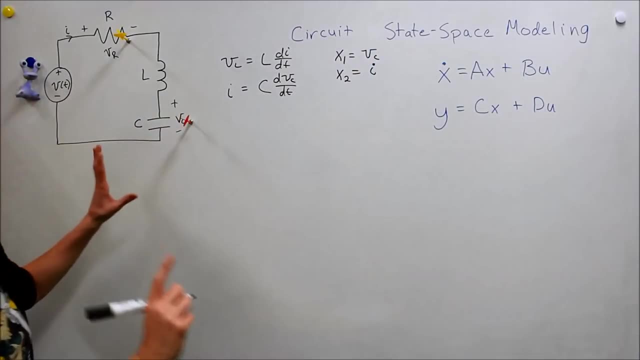 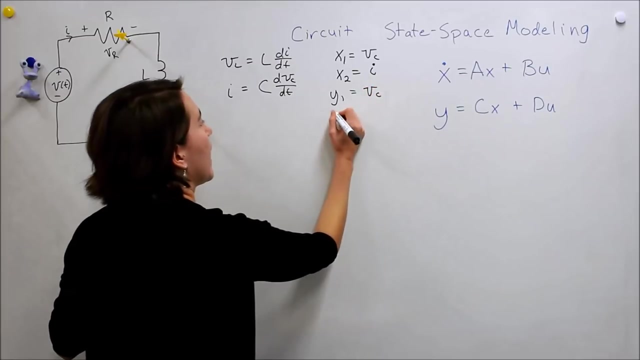 so V C and we're going to call X2.. Okay, and remember our output, so let's just write them here now. So we're going to have Y1, that's going to be V C and our Y2, what is that going to be? That is going to be. 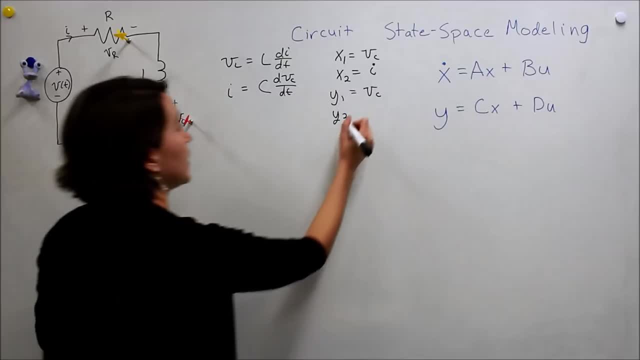 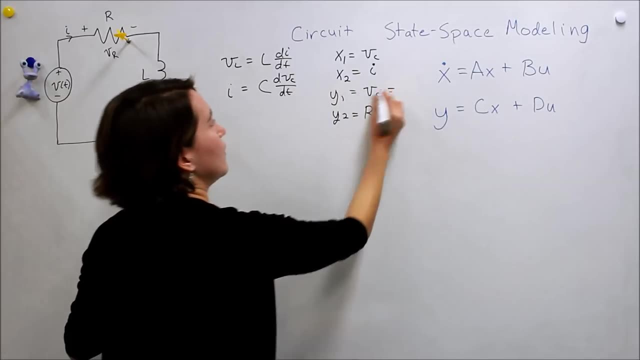 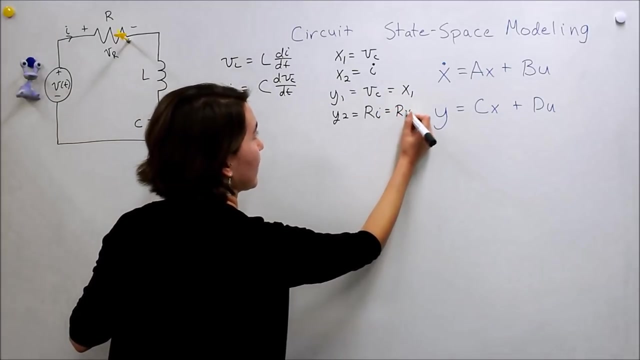 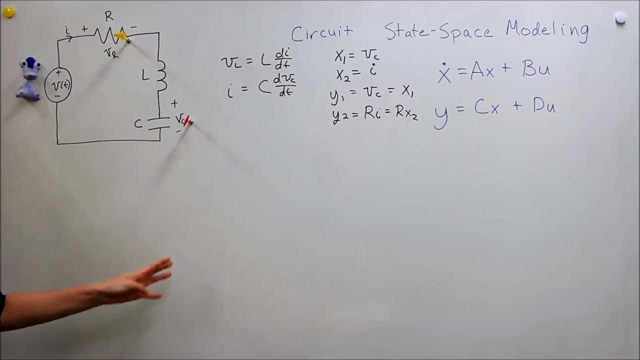 well, the current times R, so it's going to be R I, And if we change this into our state space, V, C is just X1.. And R I would be R X2.. Okay, so we've got all our main definitions And we can do some things here, And so these: 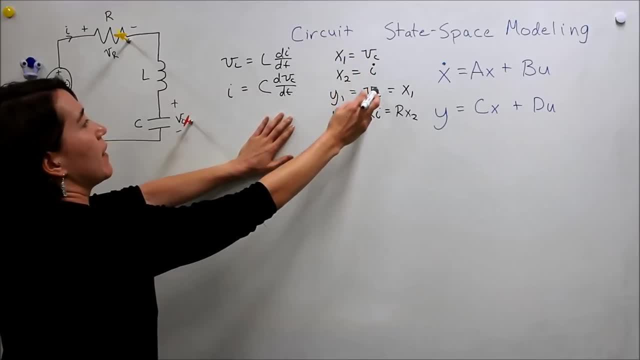 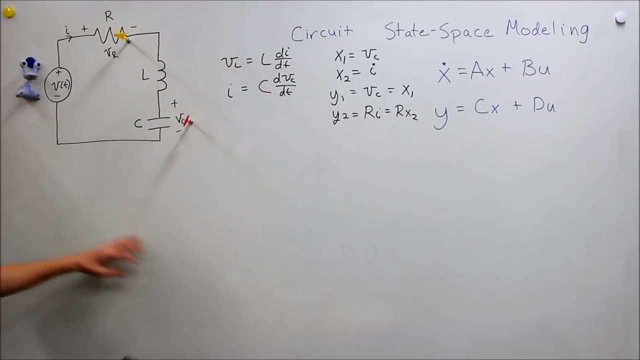 so far are all in our state. so V C, I and well, that's it, V C and I. We have this V L as well, so we actually need to find a new equation for V L. But if we look at, 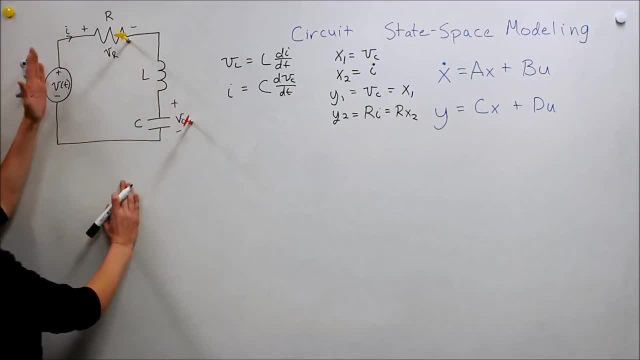 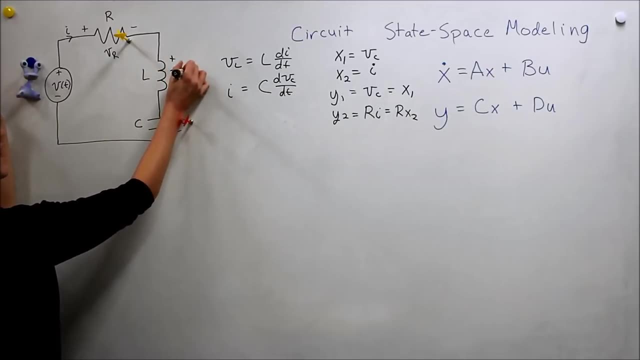 the summing up all of these voltages. so if you do K V, L- we know this is the oops, it's an L- We know that this voltage has to be equal to the sum of these voltages, So let's write that down. We have. 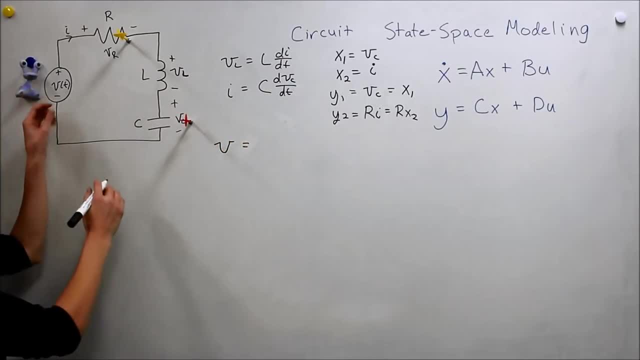 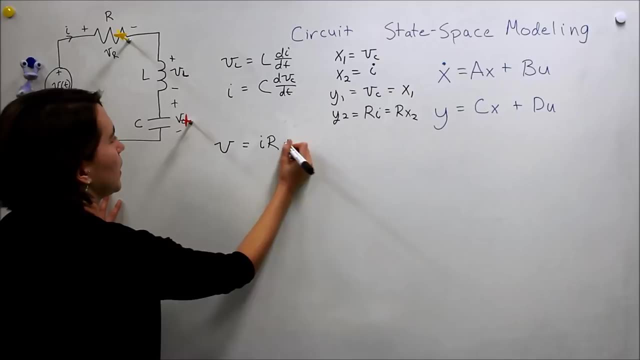 V, and I'm going to drop the of T's here again, So V, our input is equal to I R right, Plus well, V L, let's put it this way- and then plus V C. 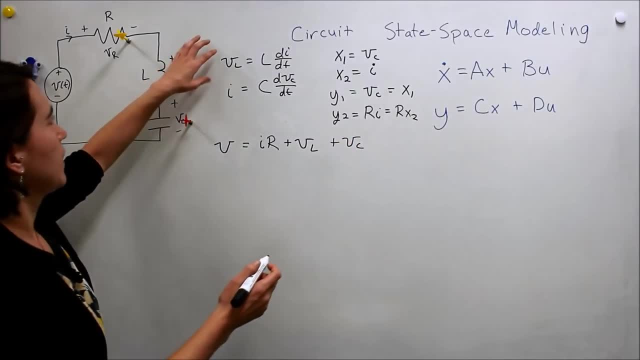 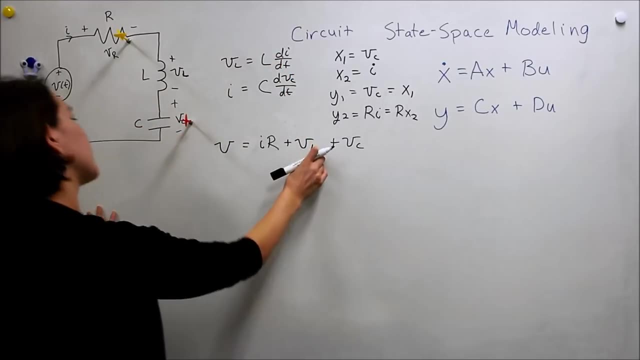 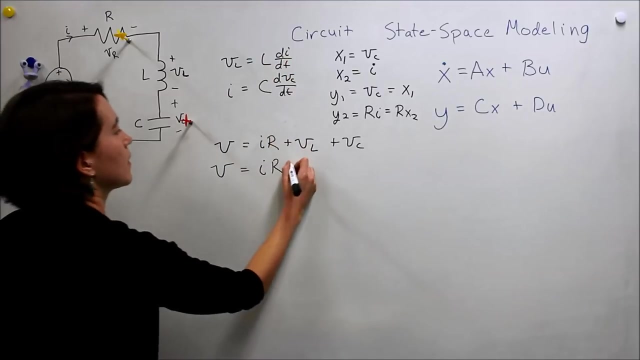 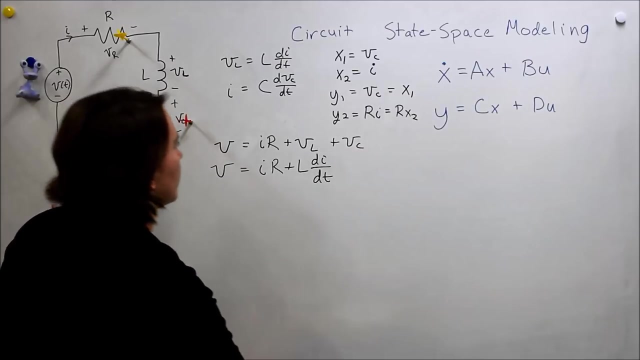 Okay, so if we put these together, we can actually get rid of our V L. So let's substitute this into here, So we'll get V equals. I R. Substitute this in plus: L, D, I, D, T, oops. 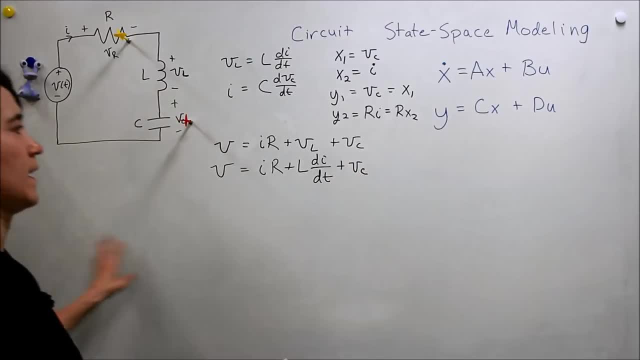 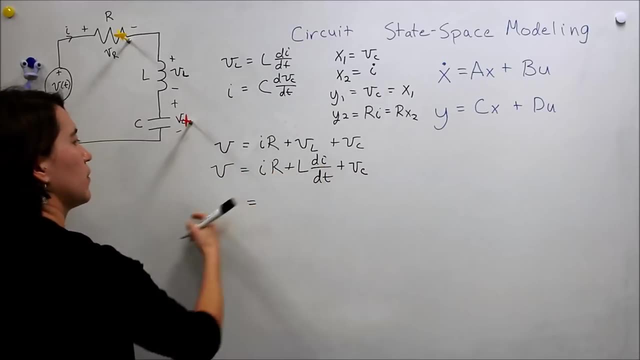 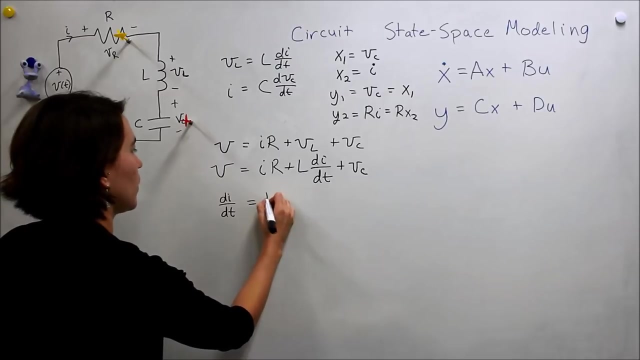 plus V C. Okay, Now we want to get D, I, D T all alone. so let's move things around and then divide. So I'm going to move this over here: I D T and we will get, so it would be one over. 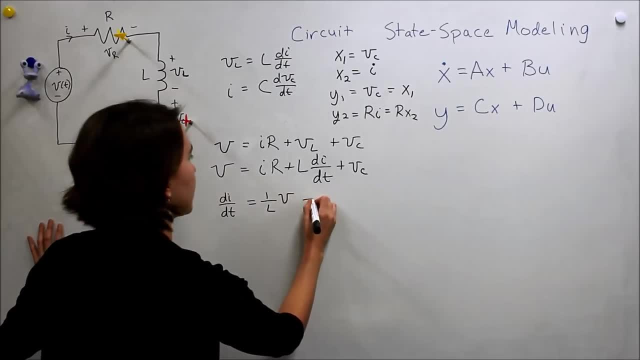 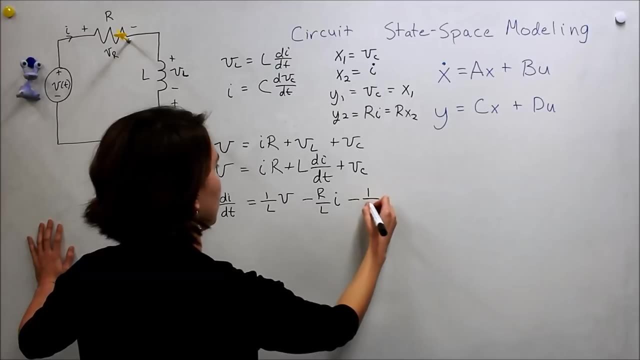 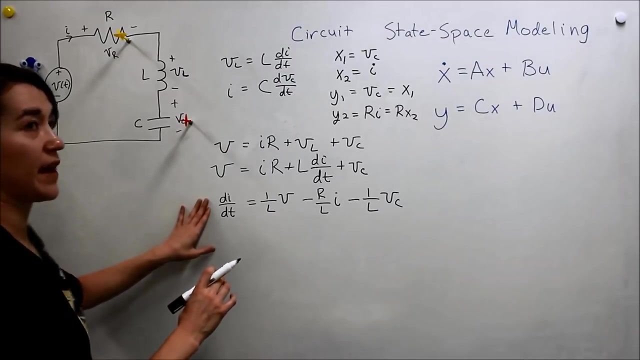 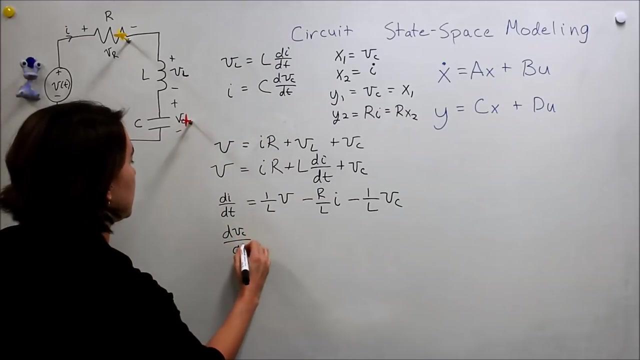 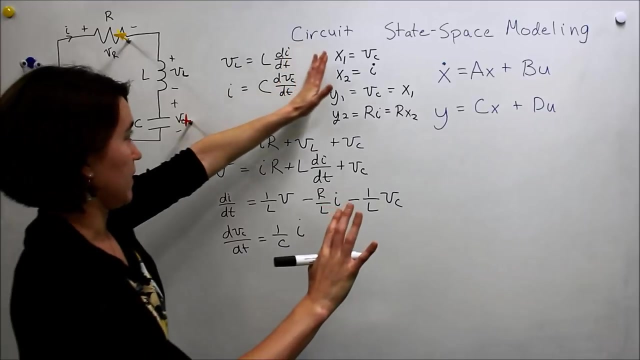 L V minus R over L I, minus one over L V C. I believe that's right. Okay, so now we have the dynamics written here And we already know this equation right. So D V C D T is equal to one over C I. Okay, so now let's transform some of these. 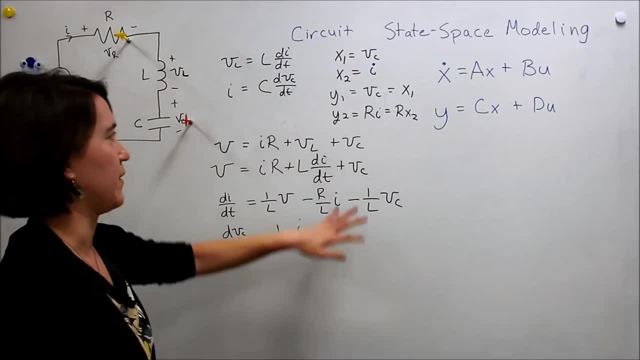 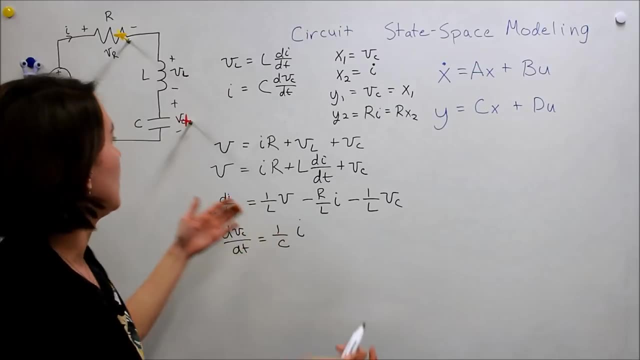 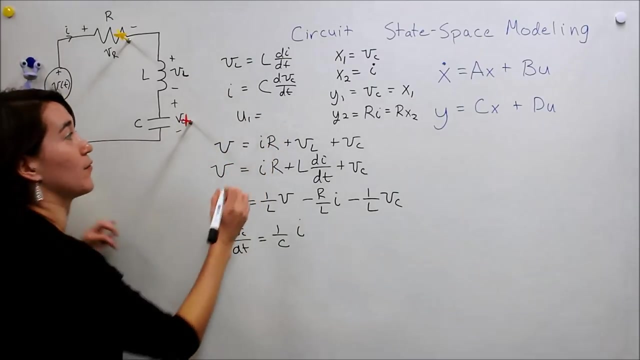 Use. instead of going in our I and V and all that notation, let's put X, X1,, X2 first. We forgot to write something down. We also need to know the input. So our input, let's say U1, is equal to V. Valerie is controlling our input at the voltage, so that's V. 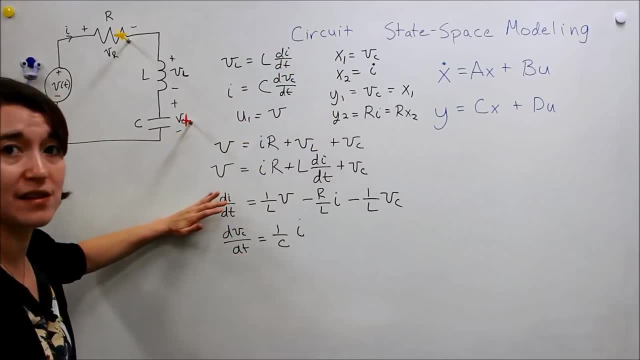 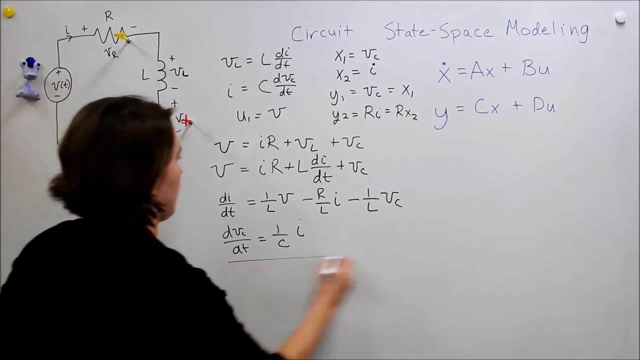 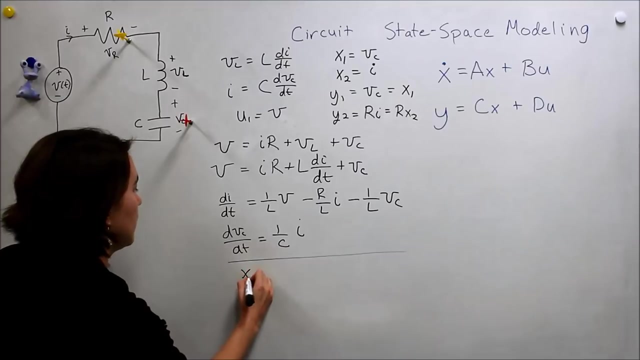 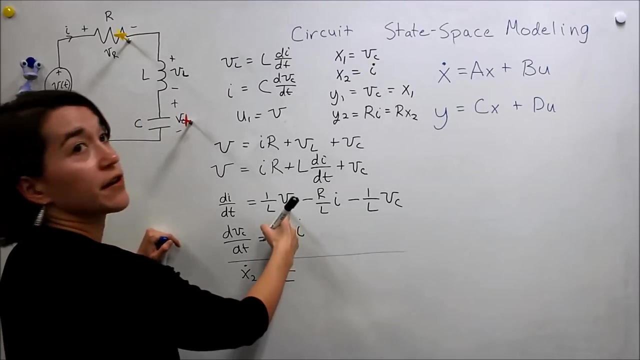 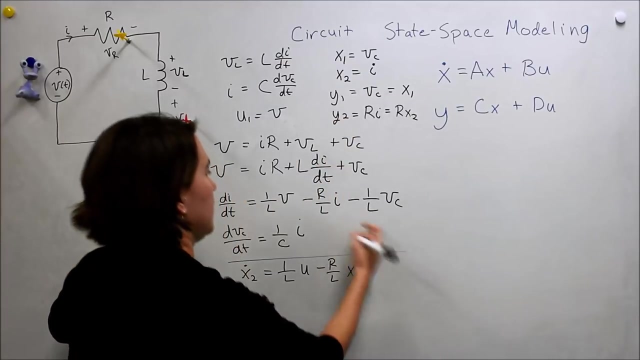 Okay, so now we have everything defined and now we can replace these two equations with our state space. So let's do that. Okay, so let's have X2. dot is equal to one over L, V, here is our input right. So U minus R over L, I is X2, so X2 here Minus one over. 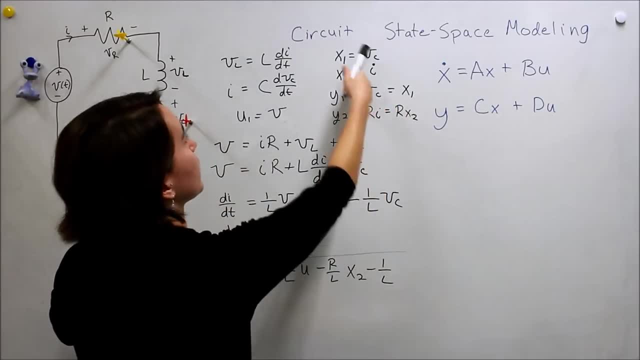 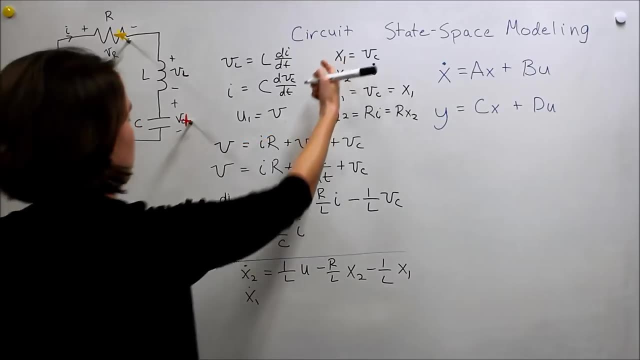 L, V C is X1.. Oh there, V C is X1.. Okay, And we'll do the same thing with this one: X1 plus V C is X1, and we have one over C and X, I is X2.. 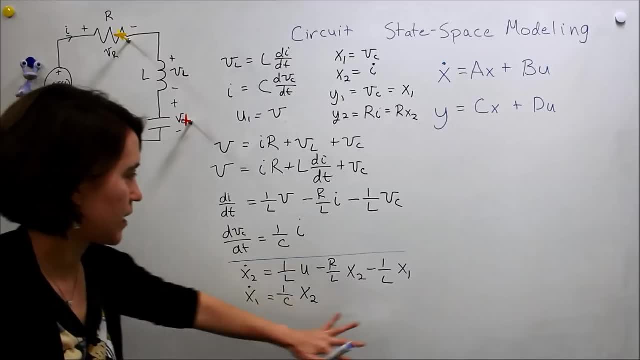 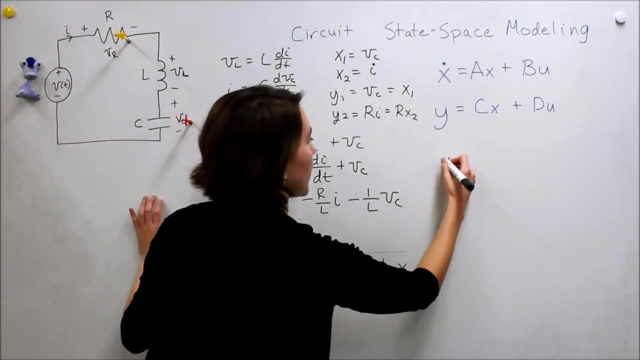 Okay, so looking at this… we can now put this into our matrix form over here, so let's move it up over here. But we'll do x1 dot, x2 dot. Now we need to figure out our A matrix and we can kinda 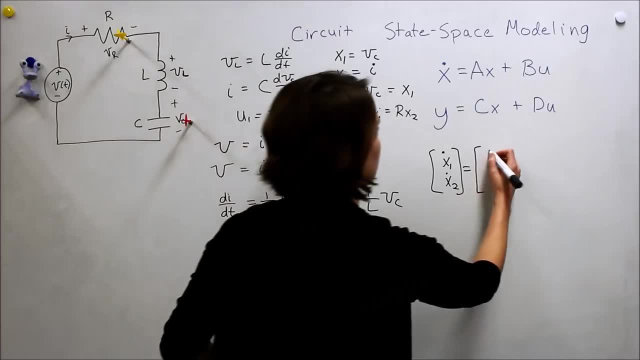 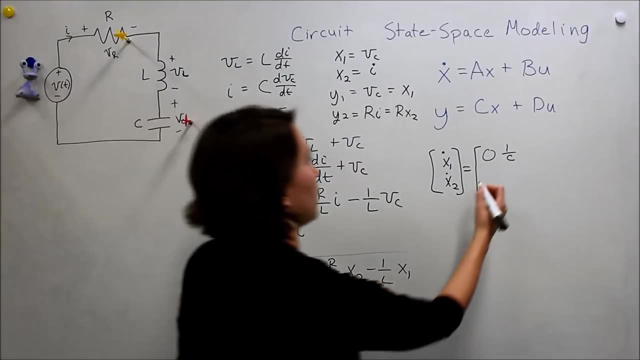 look at this one and see it only relies on x2, so we'll have a 0, 1 over c, and now we're gonna fill in this part of the matrix, so we're gonna have a negative 1 over l and then a negative r over l. 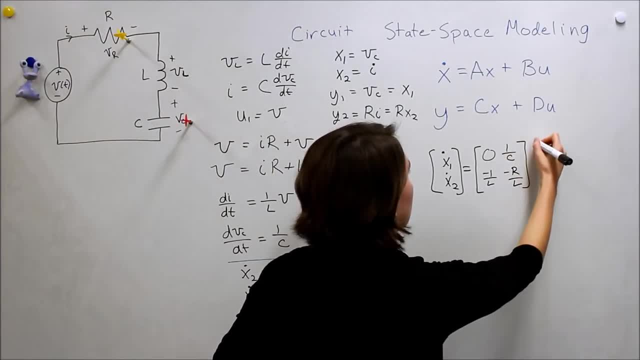 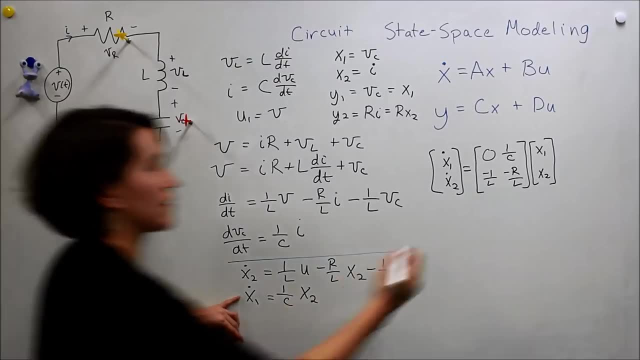 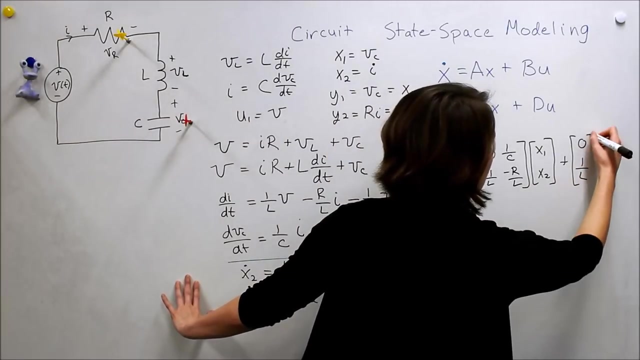 times our states x1 and x2 here And now we have to look at inputs. x1 does not depend on u. Put a 0 here, Next two, we have 1 over l times u Great. so again, here's our A. 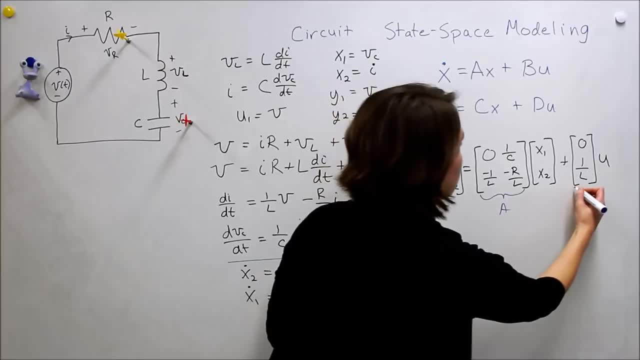 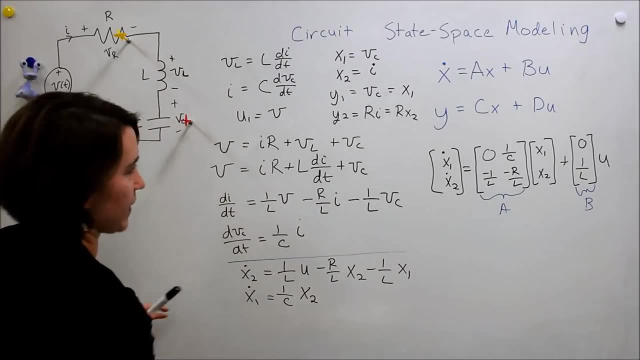 A and here's our B. Now what about y? And we have 2? now What do we do with that? Well, we've already written it here, so let's see what we can do. So we're gonna put y1.